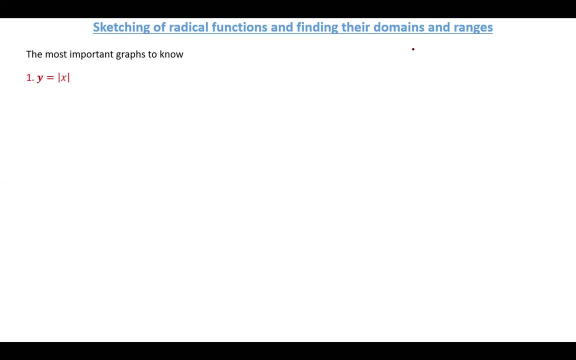 what do they imply? So when you have something like maybe, for instance, y is equal to, you know plus or minus negative one, So when you say the absolute value of this negative one, the answer will be a positive number, which is just a positive one. That's the meaning. 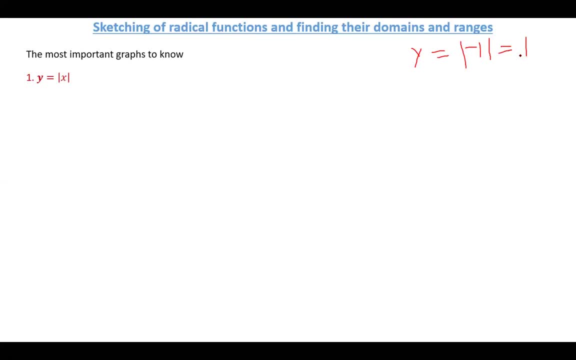 of absolute values. So in other words, the opposite of that given negative integer. It is not. the opposite is not true. The opposite is not true. The absolute value of positive one is not negative one, It is an integer. So the opposite is not true. So you need: 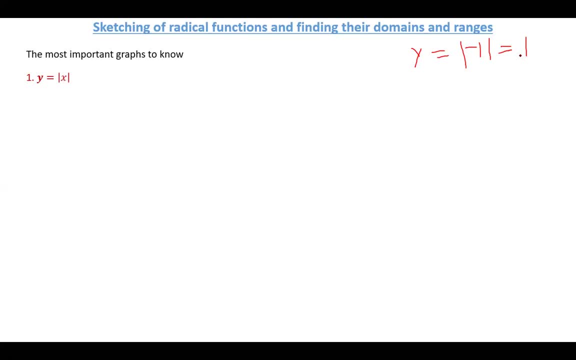 to know positive value of x. So maybe we can go to here and maybe you can just do a little bit more. Yes, Let's say the first slide we'll do with this one. We can do a little bit more. the absolute value of positive one will still remain one and then at least the. 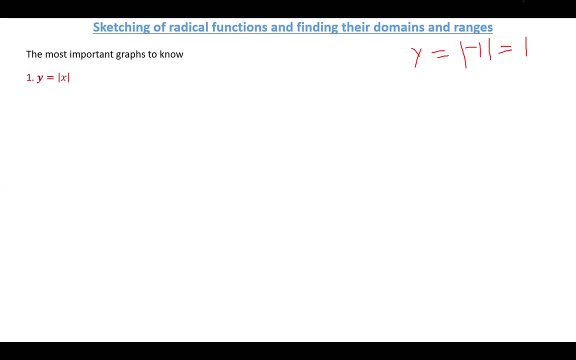 absolute value of negative one, that's one which will give you positive one. yeah, so we proceed. so the absolute value of X. when you're sketching the graph, it comes out like that. you can see that is how it comes out. so you need to master this ground, need to master this sketch. then these are the domains and the range. 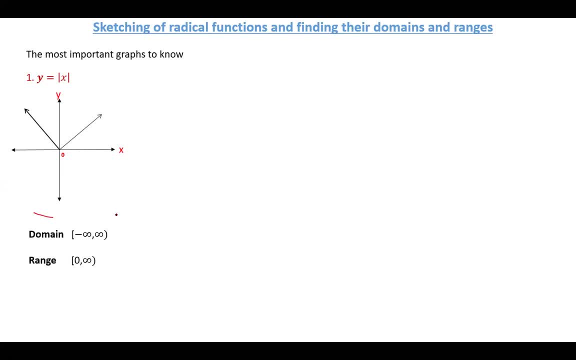 of the above graph, of this graph here since the domain. so the way you find the domain, the range, is the same way we are doing in the previous nature slide where you- you sorry, this one was supposed to be an open bracket. yeah, so for absolute value functions we should not say the domain is just the set of all real numbers. 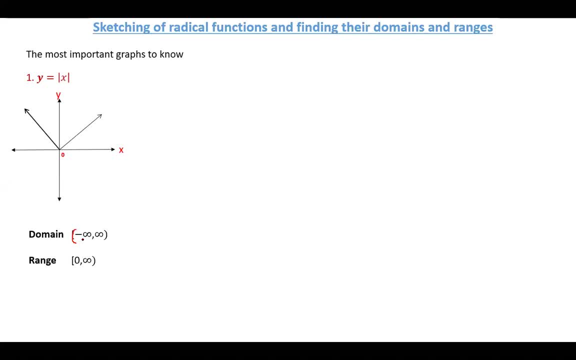 which implies that all negative integers and all positive integers inclusive, and then so. so now we talk about the range. so finding the range range- here you can see it is only on the positively and which implies that, which implies that I was starting from zero. 0 is also part of the set. then up to 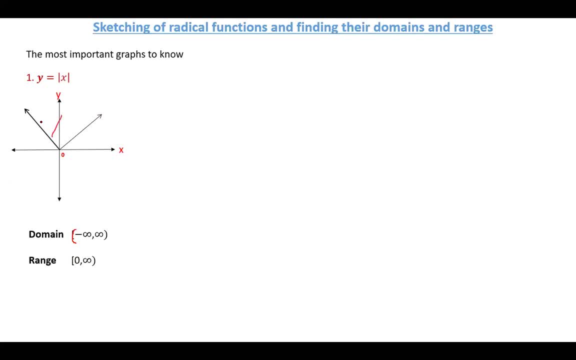 infinity, meaning we're talking about to this area, this side, only talking about this area going up. that's the arrangement. and then the range is only measured in the y-axis. yeah, one of the one, of the absolute value function has a negative outside. how does it look, or what does it look like? so, in this case, 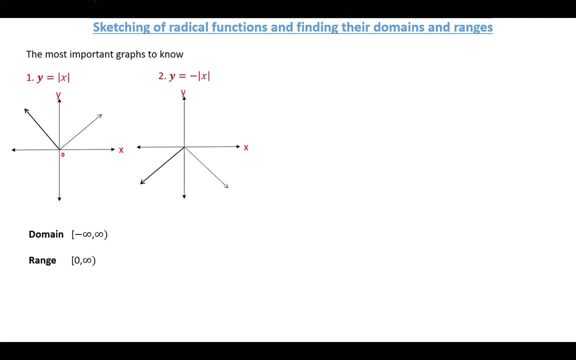 it is going to face down. so this negative here is simply just negative 1. so this negative is just the same as negative one there, so negative one there. in other words, some people call it the gradient. so when it has a negative in front there, just notice it's going to face down. and these are the domains you 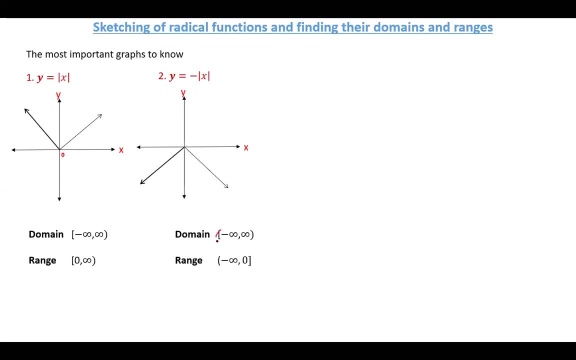 can see the domain. like I said, this is also supposed to be like that, supposed to be an open bracket. the domain, like I said, for all absolute value functions in can insert any real number. there you still have a like, you still get a solution for that. except it, they accept if there is a. 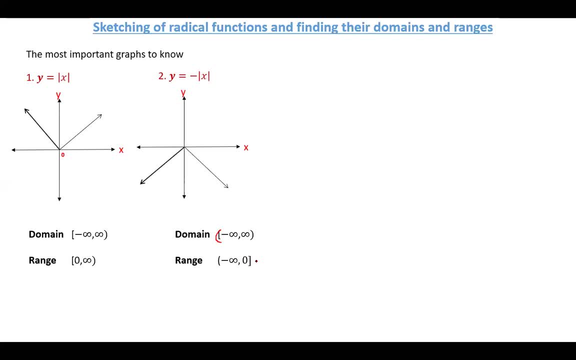 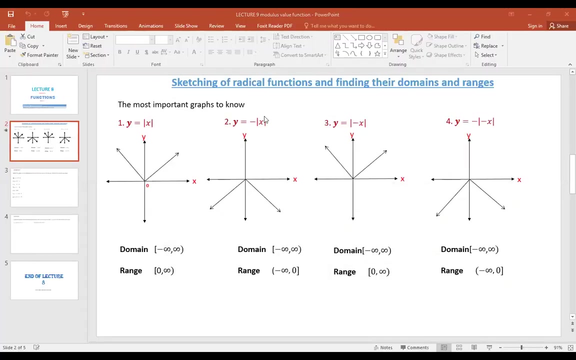 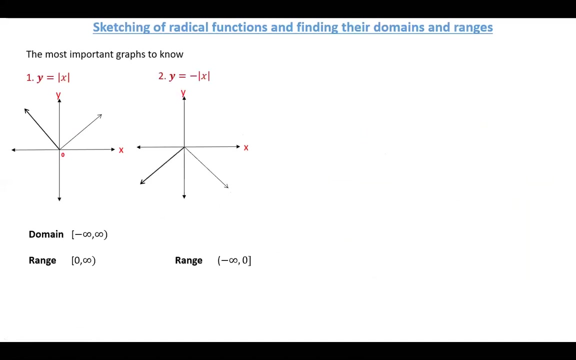 randi cope somewhere. so we talked about the range in. see that we're only talk about the y values. they are only have Y values in the negative. we don't have on in I. Okay, so let us quickly finish up this, okay, sorry, okay, yeah, so we proceed. 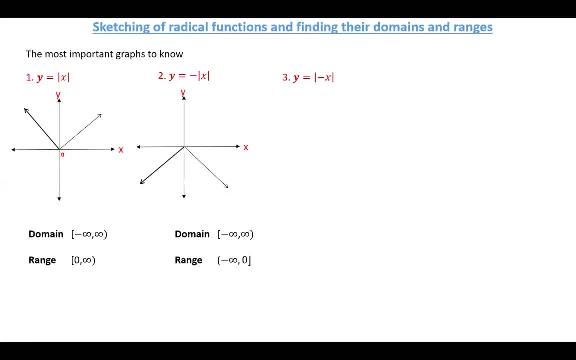 So what if you have the negative inside? Remember what I said: when you talk of absolute value, we're simply talking about the negative numbers being transformed to positive. So the absolute value of negative x will still give you a positive number. So this one. so when you look at this one here and this one here, there's no difference. 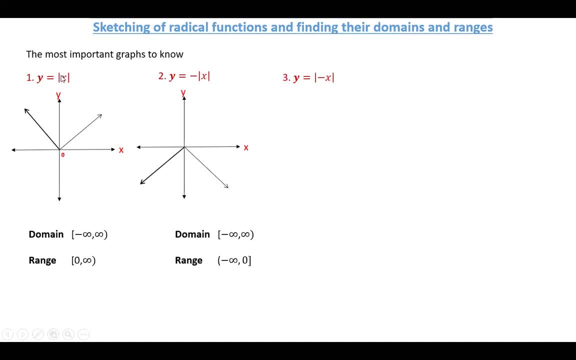 due to the fact that any of these numbers are positive. So this one. so when you look at this one here and this one here, there's no difference due to the fact that any number, the absolute value of any positive number, will give you a positive number. 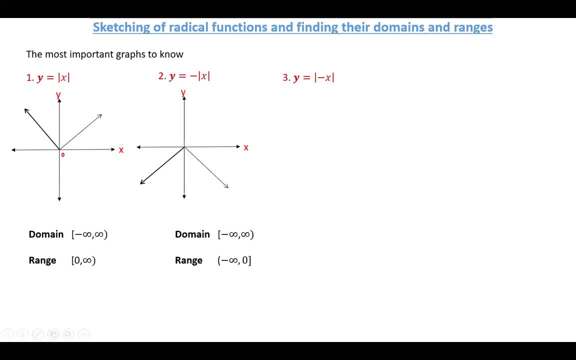 Here, the absolute value of any negative number will give you a positive number. So, meaning this, meaning this, and that are almost the same are actually even the same, So the graph will not change to just come out the same way as the first one here to. 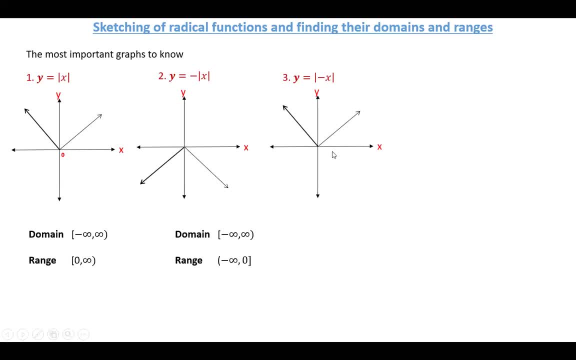 just come out the same way as this one. This is what you're seeing there. The domain and the range will still stand the same way. Remember, here there was a mistake. I just hope that I'll remember correct this, this mistake, after, after the lecture. so 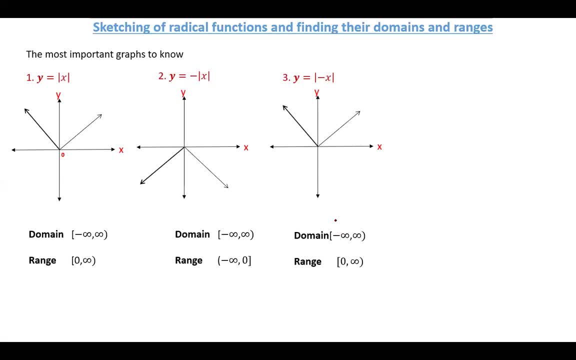 that, as I'm going to be sending the lecture slide here, is going to be an open bracket like that, So proceed. What if you have both inside and outside There is a negative, just to come out as the second one here? why? why is it? why is it? 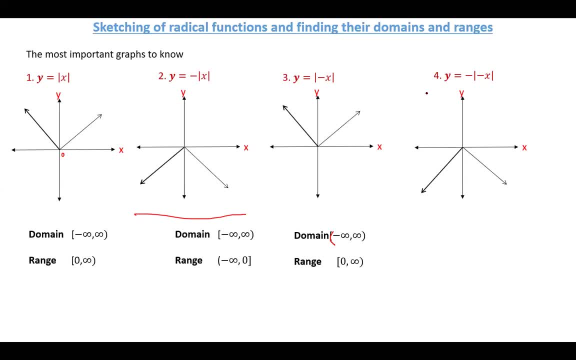 coming out as this one, Because here we, as we said, here we said to say the absolute value of any negative number: X, you will still give you a positive number. So meaning this one, the only negative number, the only negative that is effective here. 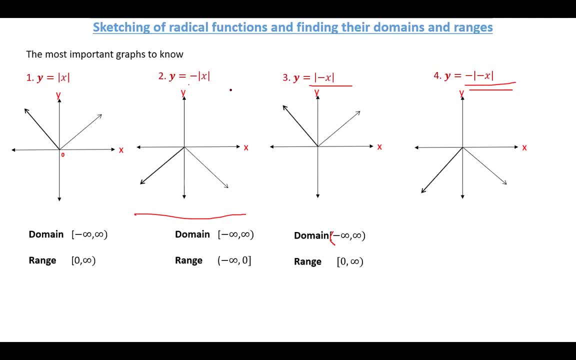 is this negative outside, which will be like this. So this is the reason why we have seen this scale. I mean, this graph and that graph are just the same, So the range and the domains will be the same. So here it's also supposed to be an open bracket. 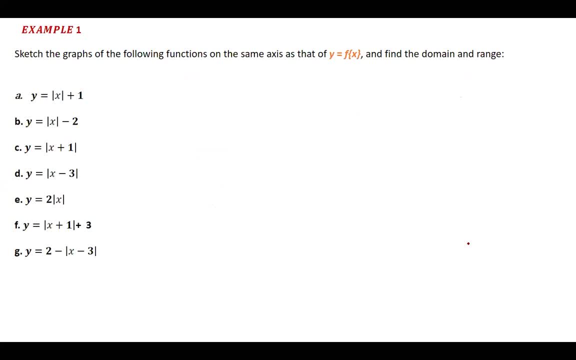 Okay, we proceed. So let us now try to take a look at these examples. Ah, The first example: A, B, C, D, up to G. So after doing this, I'm pretty sure, and I'll know, and I'm sure to say, you guys will be able to sketch any given graph. 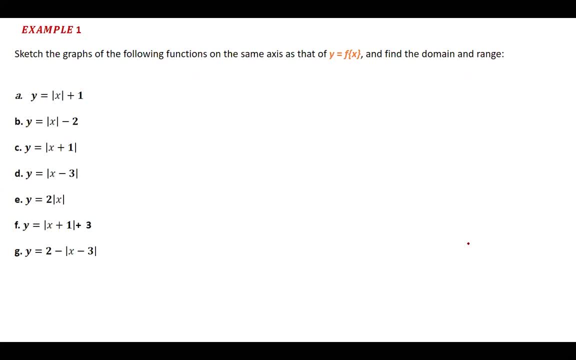 And there is also an exercise at the end of this slide which should be requested to answer and submit before Thursday. So the first one here. Yes, So the first one here. When you look at this one, you have the absolute value of X plus one. 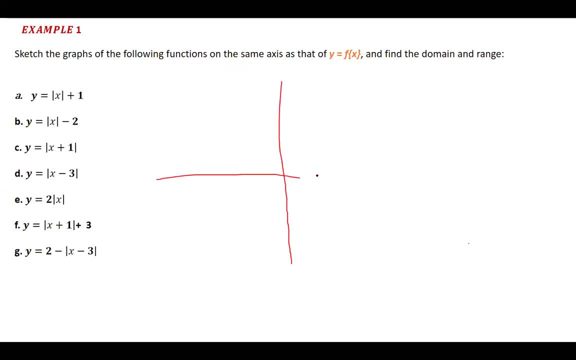 So how does that come out? It's going to come out as it's going to be, like this: Yeah, So the absolute value of X. we know that it always comes out like that. This is how the absolute value of X comes out. 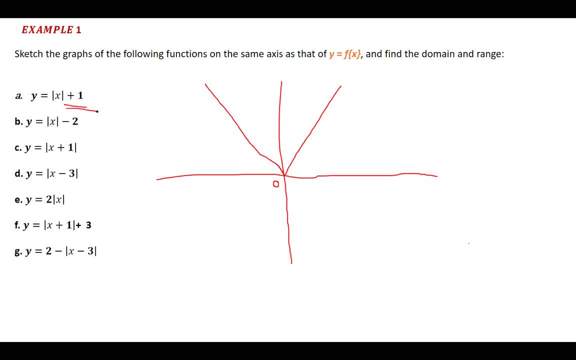 Now, if there is a plus one here, Then it's going to be like this: If there is a plus one, it simply means that you are going to. if there is a plus one there, simply means that we're going to shift in the Y by one. 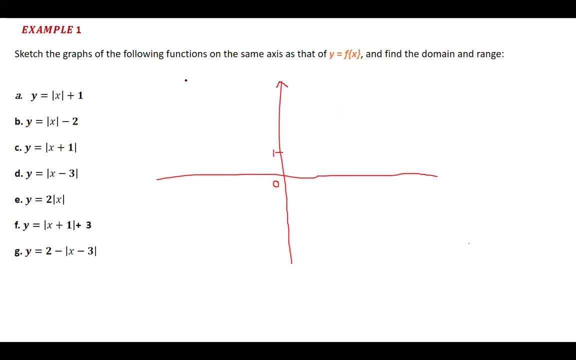 So we're going to shift by one in the Y, like that. So this is how it's going to come out. Okay, So it's just as simple as this. Then the domain: the domain will always be the same, as I said, or just a set of all real. 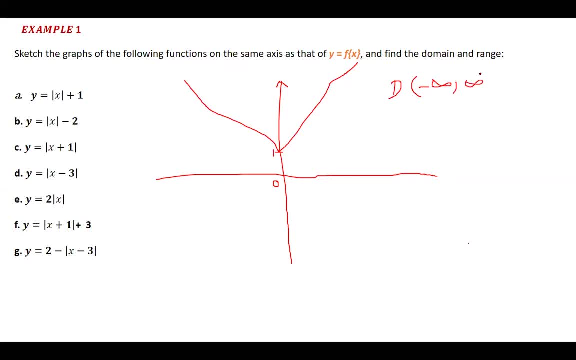 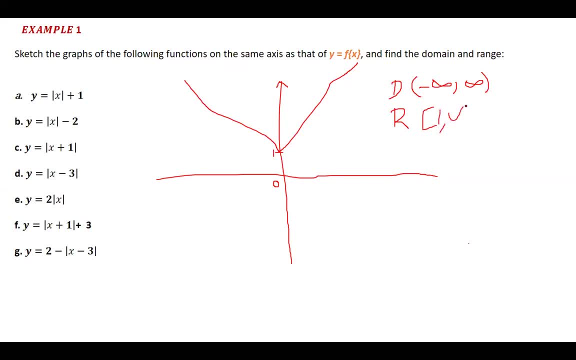 Okay, Okay, Okay. This is Then going up. we are starting from one going up, So starting from one going to infinity. So this is the domain and that is the range. I don't know what else is remaining, So here, 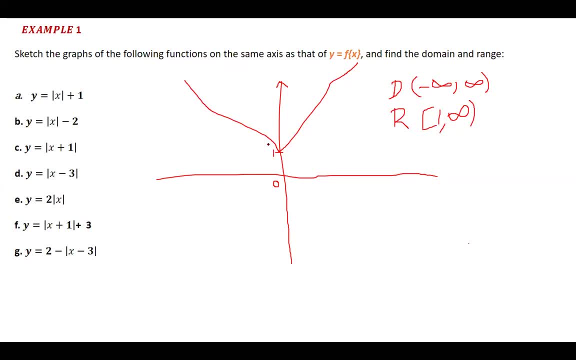 Yeah, So on this one, here is the range. This is the range. Yeah, This is the domain. So I, this is straightforward, this is how you sketch it. so if you want, you can use this table of values. if you just want to be at least a little bit accurate, you can use the table of values to sketch. 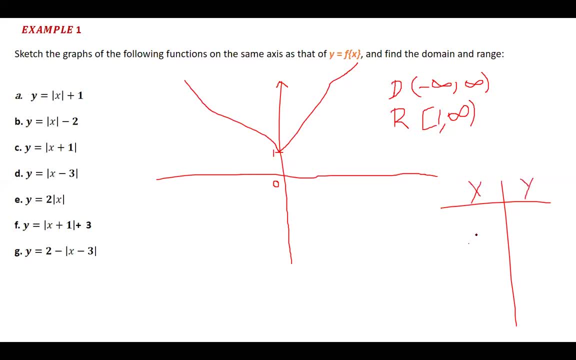 use the table of values to sketch, then you plug in some numbers there and then you can use the table of values to find the answers. so let us now move on to the next question, because this one is done. they are simple. i don't know why most people find difficulties when it. 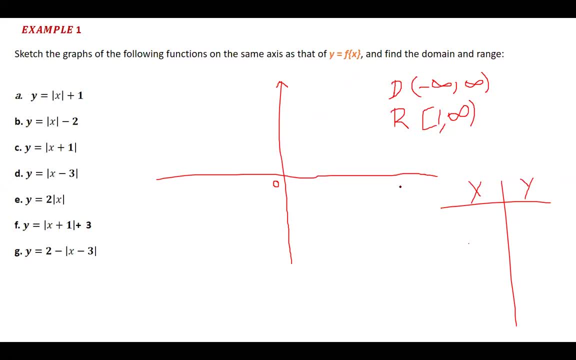 comes to answering such questions. so we move on to this one. so this one is just the same as this. the only difference is that this one is a minus two. so if there's a minus two, it means that it's going to cut the y-axis at negative two, like that, and then it will still face up. 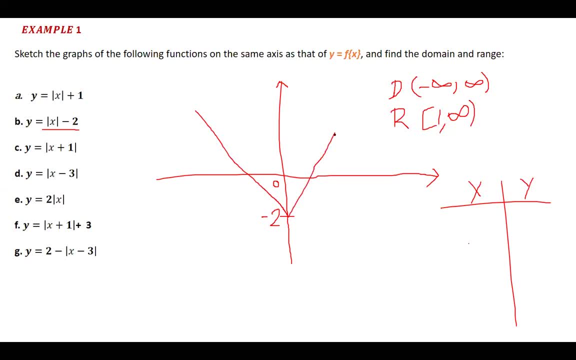 to still face up like that. so at one point, i'm going to show you how to solve these same equations in order to find this value there and that value there, yeah, even this value there. but for now, i want you to first know this, so that the next, actually i'm going to show you in the next slide, in the next. 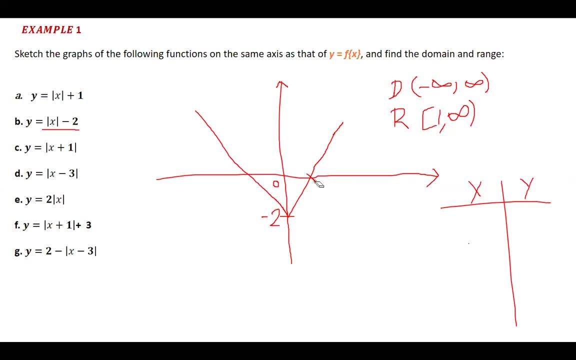 lesson that we're going to have, since we're going to be solving uh equations involving absolute learning functions, including equations involving the radicals. so this is how it comes out. now somebody might be asking: how do you solve this problem? so i'm going to show you how to solve it. 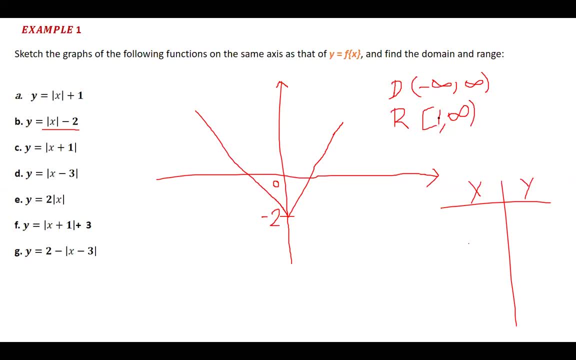 okay, so let's get started. okay, so how should we solve this problem? so how do you find the range and the domain? the domain still remains the same. and then the range: here we have negative two, meaning we are going to have negative two going up to positive infinity. 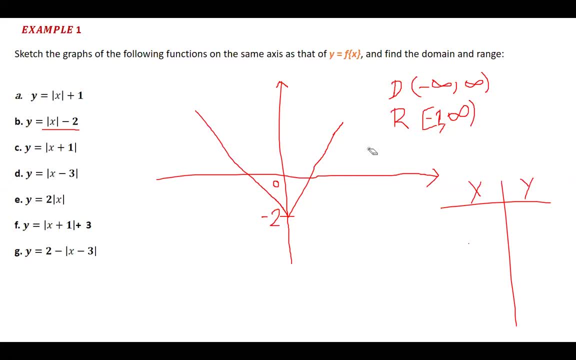 it is just as simple as that. okay, wow, so we proceed, we go to C. so we proceed, we go to C. we want to see, so see, saying the absolute value of X plus 1. so here what you do is remember to are doing yesterday on radicals, so you equate to: 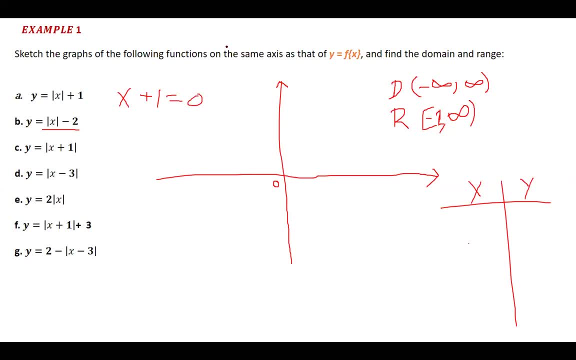 this to 0, then you find the value of X. so the value of X there will be negative 1. so if the value of X is negative 1, what do you do you? it simply means that the the graph, rather they, yeah, they got the graph that you are. 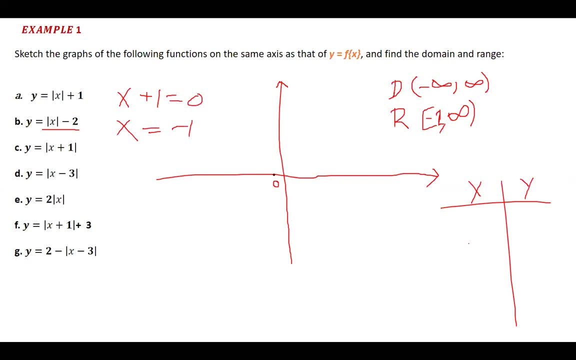 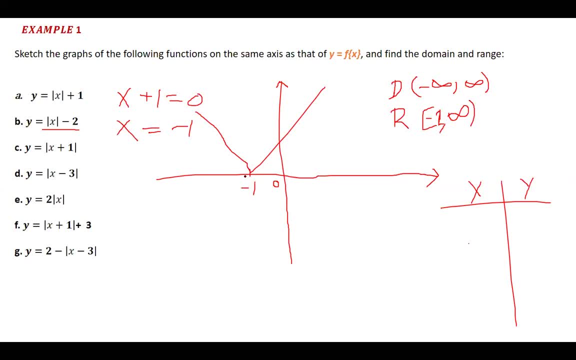 domain and the range: the domain will still domain and the range- the domain will still remain the same. the range here will remain the same. the range here will remain the same. the range here will be. we're starting from 0 going up, so be, we're starting from 0 going up, so. 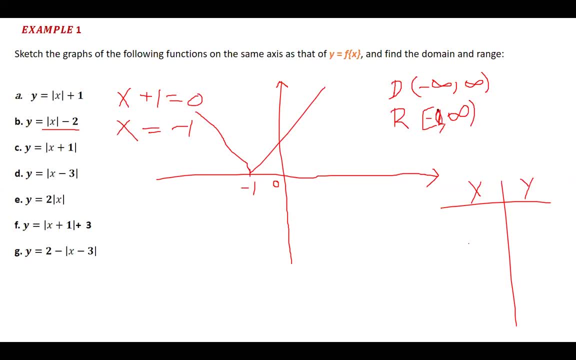 be. we're starting from 0 going up, so starting from 0. so this is going to be starting from 0. so this is going to be starting from 0. so this is going to be 0. can you just delete it and write 0? can you just delete it and write? 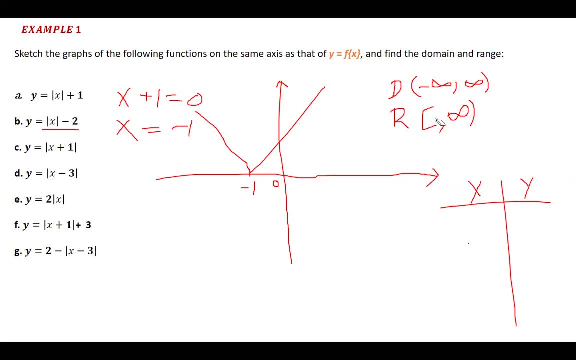 0. can you just delete it and write something else, something else, something else? she's 0 comma infinity, like that. so these: she's 0 comma infinity, like that. so these, she's 0 comma infinity, like that. so these questions are just as simple as. 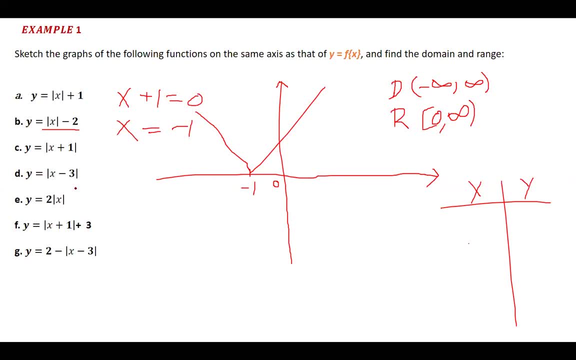 questions are just as simple as that. you don't need that, you don't need to stress for you to answer them. all right, we proceed. let us do: y is equal to x minus three. so for y is equal to x minus three, you equate your x minus three to zero. 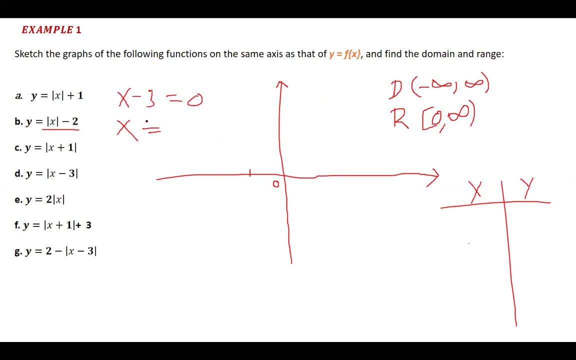 so x minus three, zero, such that your x value will be positive three. and then this is going to be one, two, three. okay, so this is where the graph is going to turn. uh, it's going to tend from here. so we draw now the k. it's going to be like that. 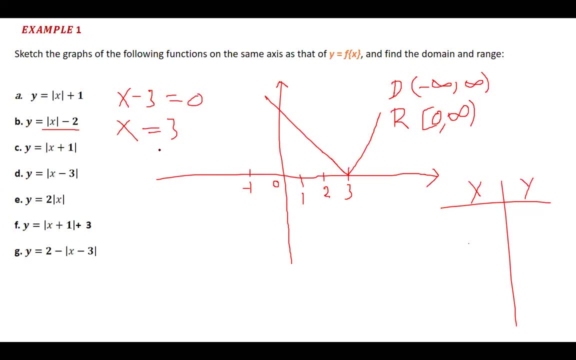 okay, so when you try to replace zero where this x, you discover that the value of y will still be negative three. then, uh, the absolute value of negative three. this is the three that you are going to have there. okay, so what is the range and what is the domain? there is? the domain will still remain the same. 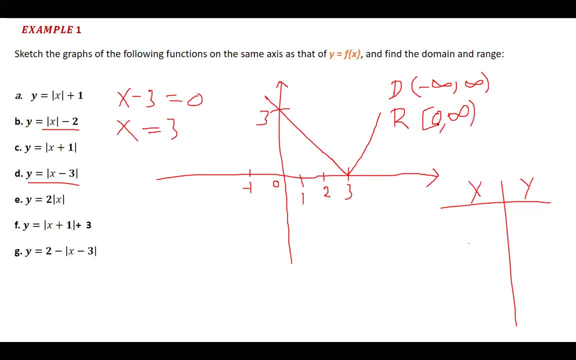 the range will start from zero to infinite, like that, still the same. okay, we proceed. so these questions are very simple and straightforward. i don't know why a lot of people stress when it comes to answering them, so i'm just going to go ahead and answer them. 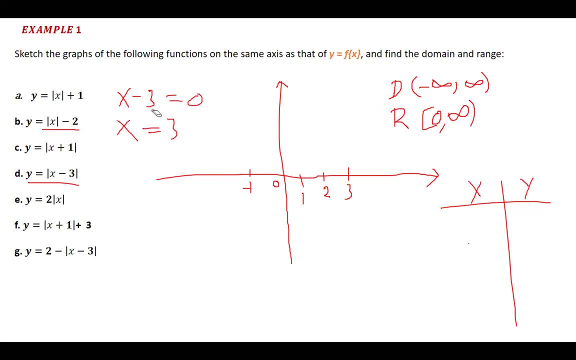 they're very simple, okay. so let us move on to e. so e is saying y is equal to 2x, so that's two in front of the absolute value. of x is just, like i said, some people call it the gradient. so, since it's positive meaning, our 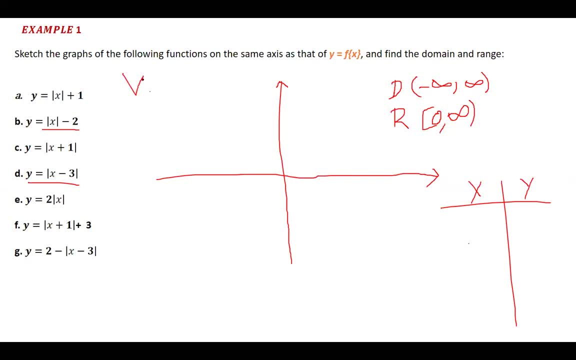 curve is going to face upwards. it's going to be like that. and then uh for numbers, uh, rather for functions which have a gradient greater than one or less than uh one. you normally do what you normally just use this, uh, the table of values, where you say you put 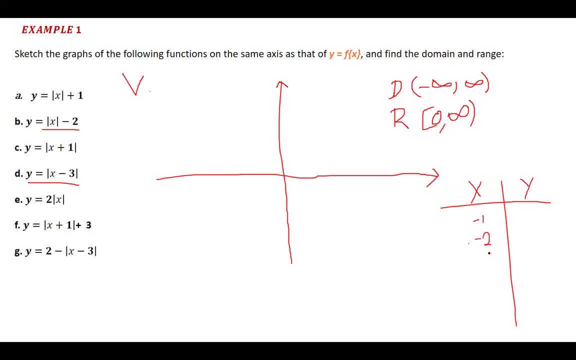 negative one, you put negative two. you put your zero, you put one, you put two. so you put negative one. while there's x there, you still have negative one. the absolute value of negative one is positive one times two. there you get your two. you put your negative two there. on the absolute value of x, you get positive two. 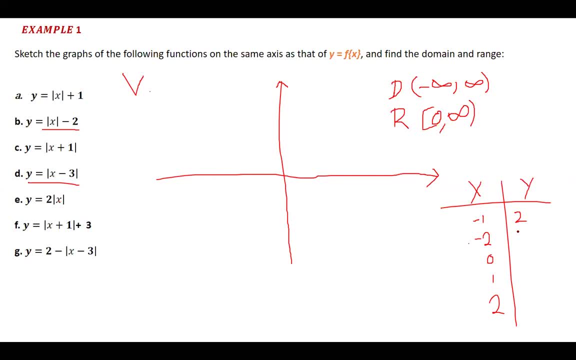 positive: two times two, you get four. when you put zero, you get zero, because zero times two still gets zero. when you put one, you get two. when you put two, you get four. so you can put your numbers there. you have to put your numbers there. Have one, two, three, four. 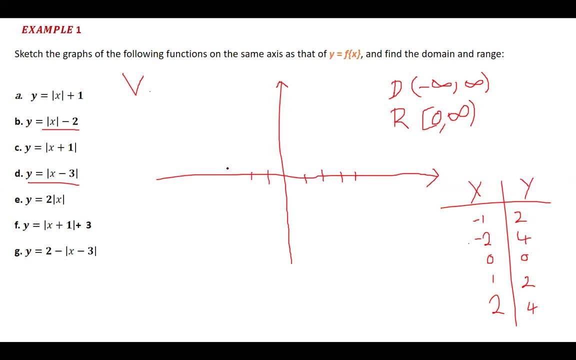 Have one, two, three. Okay, Then apart from that, yeah, apart from that, we move on to the Y Y- we have two, four, zero, two four. So you can just put this: two four, Two, four. 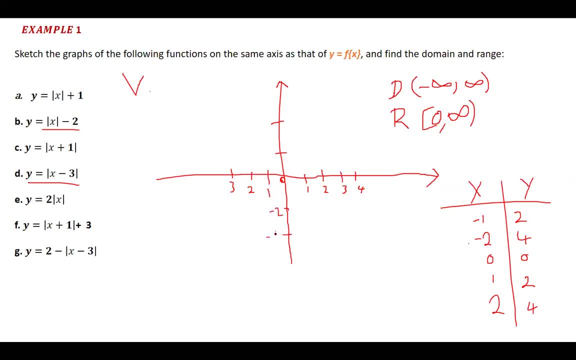 So you have negative two and negative four. Yeah, Two, four, You have four. All these are negative numbers, by the way. So we say negative one, two. We have the point somewhere there. We have negative two, four, negative two, four. 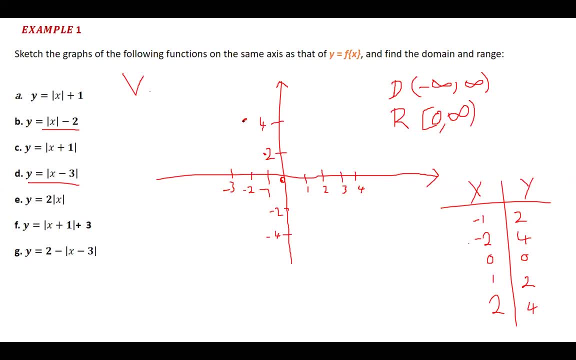 We have the point being somewhere there, So connect it like that to the center. Okay, Here on this side you have zero comma zero there. Then you have one comma two. One comma two, the point is there. Then two comma four, the point is there. 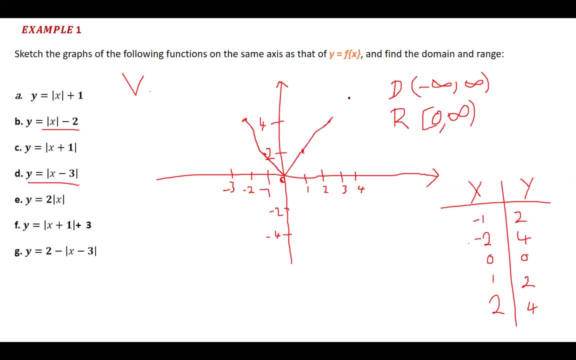 You also connect the two points. like that You can even extend it. You have drawn Rather, you have sketched: This is E, What is the domain and what is the range? So the domain: there is simply the same thing here. 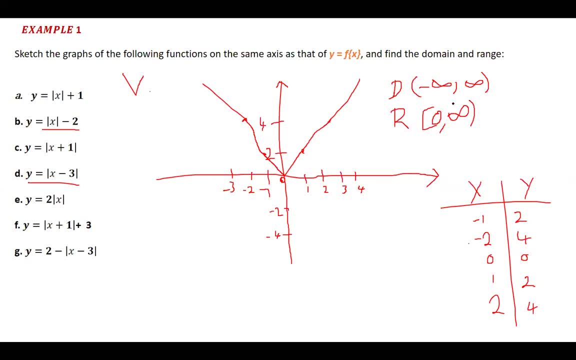 It still remains the same. And then what is the range? The range there? the range will begin from where? From two. Sorry, The range will begin from zero. to just remain like that, Because when you replace zero there, Oh yeah. 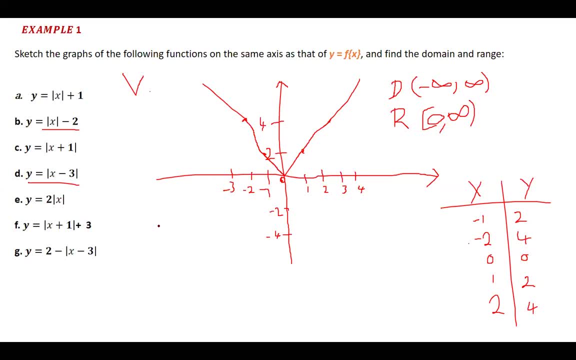 When you replace zero there where this X, you still get the zero. Zero times two to get the zero. So these will still remain like that. Okay, So these questions are just very simple. They are simple. I don't know why people face challenges when solving them. 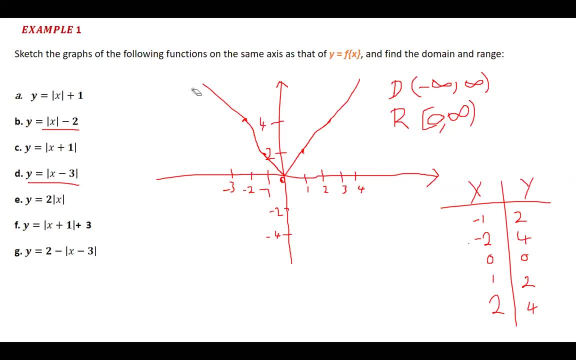 So let us also, let us finish the last two, Okay, And we call it a day for today. Tomorrow we'll do, we'll be solving equations involving these same absolute values- Sorry, not tomorrow, but on Thursday. And then we also do quadratic functions. 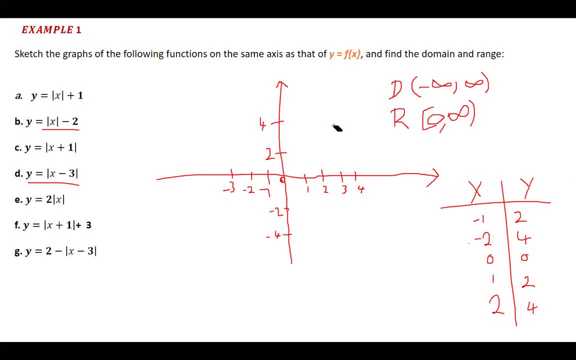 Then we're done with functions. Yeah, So, so that next week Monday we'll begin logarithms And we also do other Other things? Yeah, So, what else? Oh, I mean, which other question here? So we do this one. 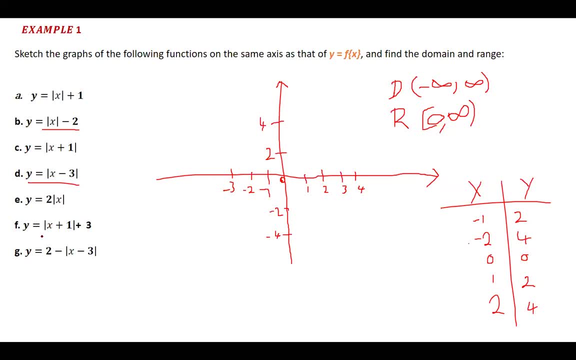 Yeah, I want to do this one, And what I'll do is I'm going to do this If the new guys are: leave G as part of your exercise, Okay. So we say I mean it's saying Y is equal to. 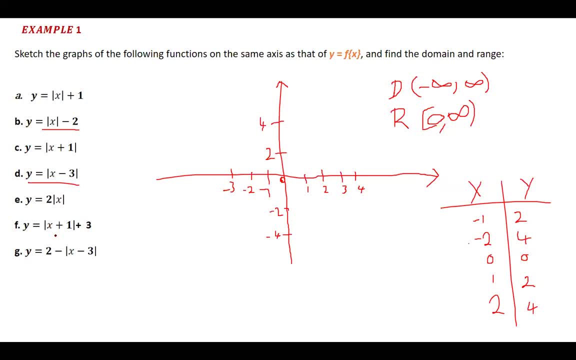 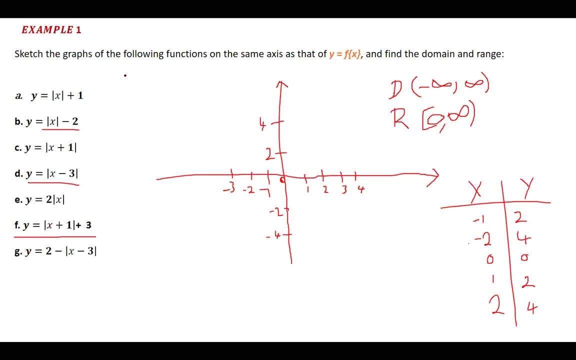 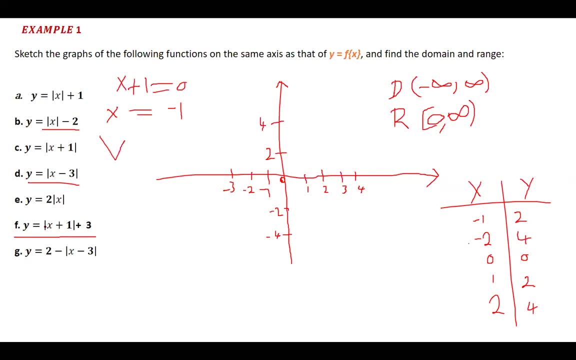 Okay to be like this, since we have a positive one in front today and then we have a positive three, so positive three is somewhere there. so the cube is going to be bending at this point, so i'm going to have something like this. yeah, something like that. 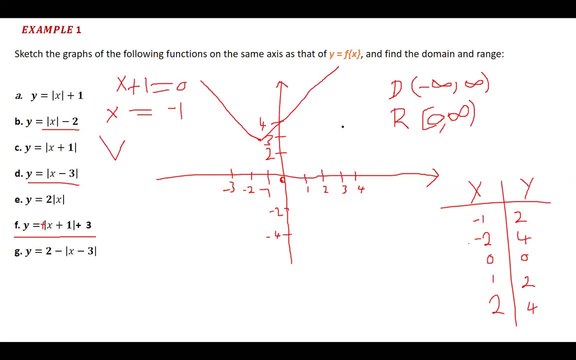 okay, so this is how you do the sketchings. they are very simple. there's nothing that is so difficult in just in sketching these things. they are very simple and straightforward. so now i'm going to add g to be part of your. anyway, let me just do it for at least for clarity sake. 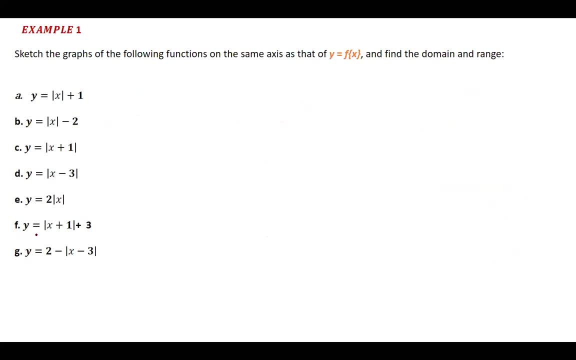 i know some people have asking themselves: how has he done this one? so let me do also g. so g is going to be like this: so we have two there, a positive two. so it's going to be like that. i'll put two there. then we have: when we get x plus three, when we equate x plus x minus three, sorry to zero. 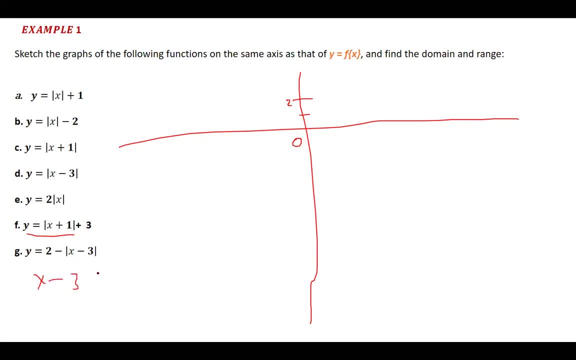 x minus three. when you equate this to zero, you discover that your x would be nothing but equal to positive three. so meaning it's going to, it's going to be at positive three. so meaning this point is the turning point for our graph, i mean for our, for the lines that: 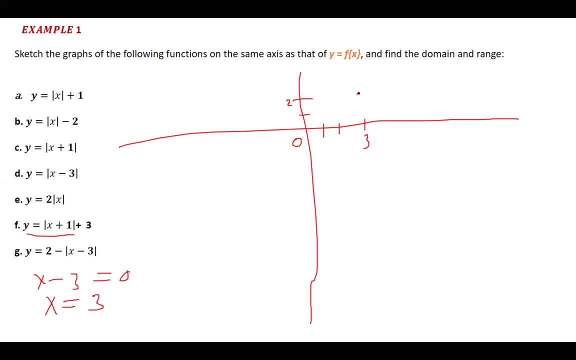 are going to draw and then is it going to face up or down? the facing up or down is determined by the sign which is in front, and in this case we have a negative meaning. it's going to face down, yes, so when you try to put a 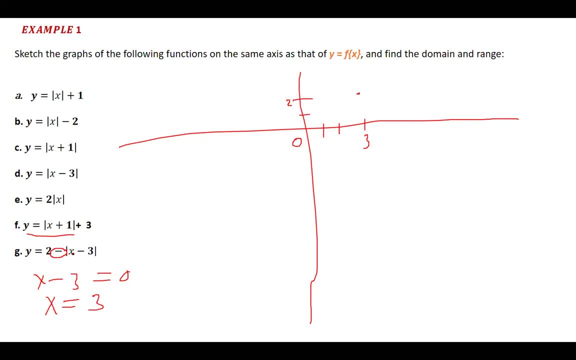 zero. where this x? there you're going to remain with three, so it's going to be two minus three, which is negative, negative one. so it's going to cut the y axis at negative one observed, and then we can also put a zero there. not positive, negative, undefined. 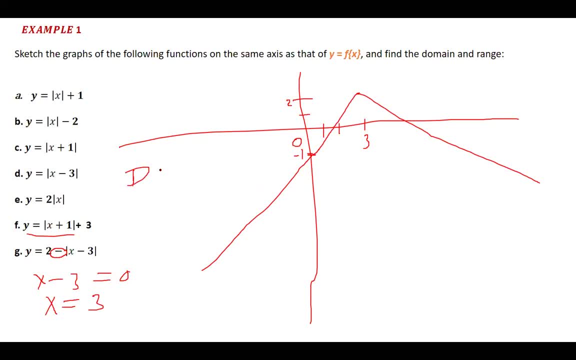 and that's how 6 goes. it's electrons, do you understand? so it's a parliament. it's zero, it's flat, very dense. how does it work? put it denoted by dance about what it's going to do. so this allows you to put a Ira to the sabbath. so if, if you can see those dominoes, which is the range path, if you can see, 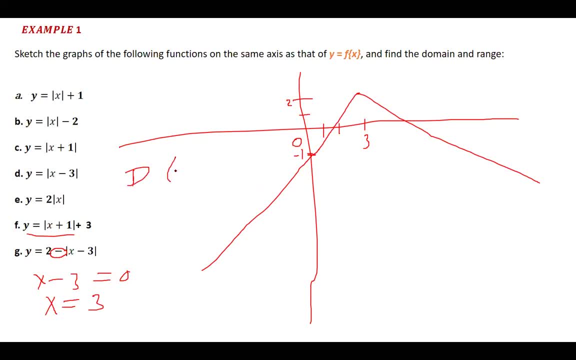 domain will always be the same, except in radicals. so it's going to be like this. then what is the range? so the range in this case is going to start from two, actually to not start from. we'll start with the negative infinity. that is, the negative infinity up to where, up to 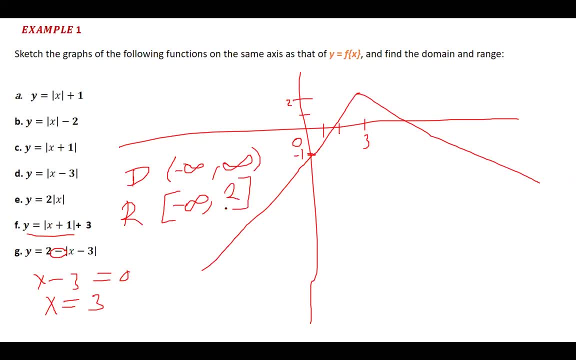 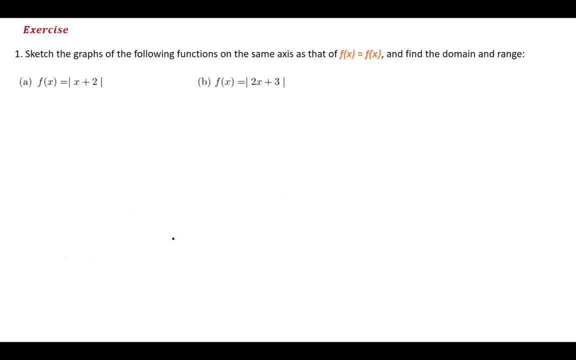 two, this one is not supposed to be. this bracket supposed to be this. yeah, i think we are now done. this was the last question. it is done. so this is the exercise that i prepared for you. i want you guys to do. i've stopped putting many questions because 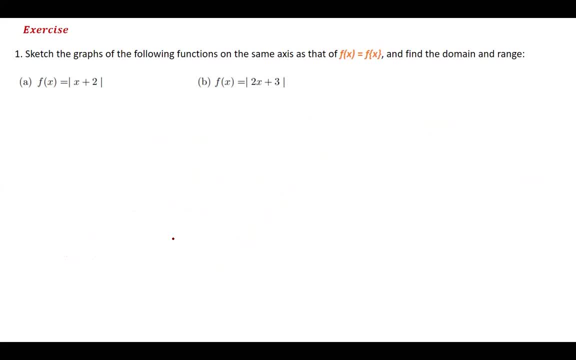 i think most of you are feeling lazy to answer them and hence you are not submitting your way. so please, for this one, i need it. i need to see how you are, uh, how, how you are understanding these things, if you have understood or not. all right, thank you very much. 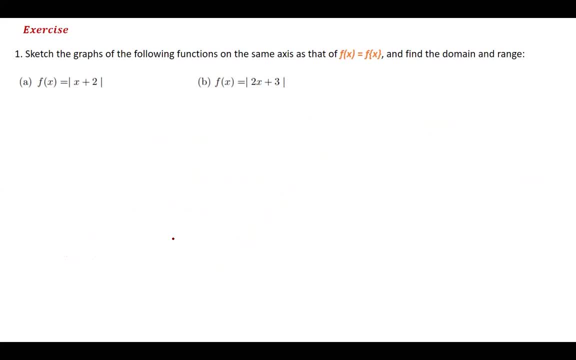 if you have any questions you can ask. i'm giving you this time to ask questions. first of all, please say hello to the audience in the audience. okay, it seems like everyone has understood. so what we're going to do now is that i'm going to end the meeting and then please make sure that you do the exercise. i'm going to send this slide.